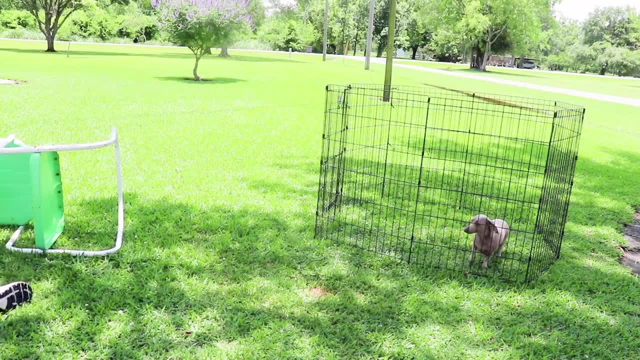 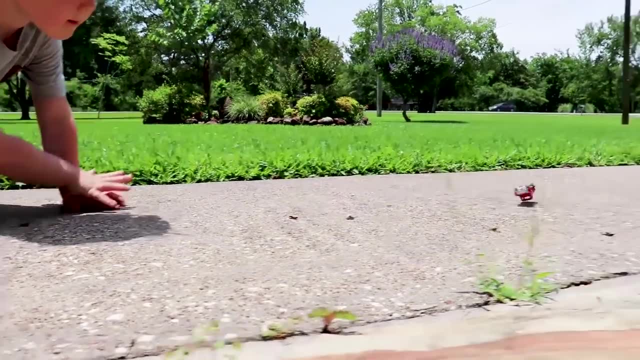 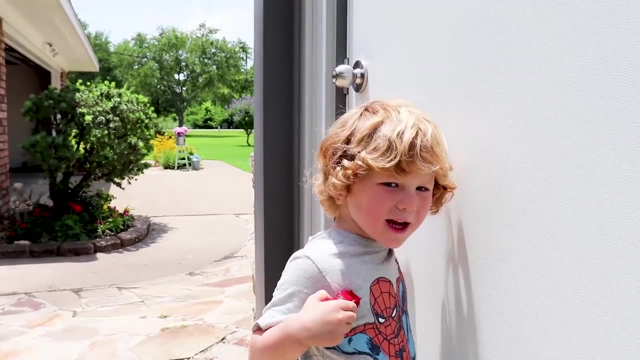 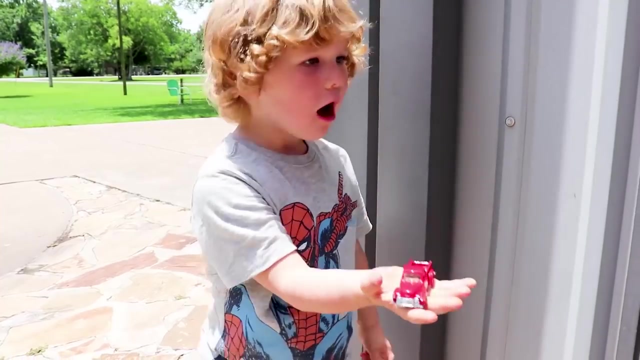 Ah, a white car Boring. Oh no, this is Pokemon Man. Let's see what's in the shop. Hello, anybody there? Oh wait, we got a customer. Yes, can I help you? My car is broken. You can fix it. 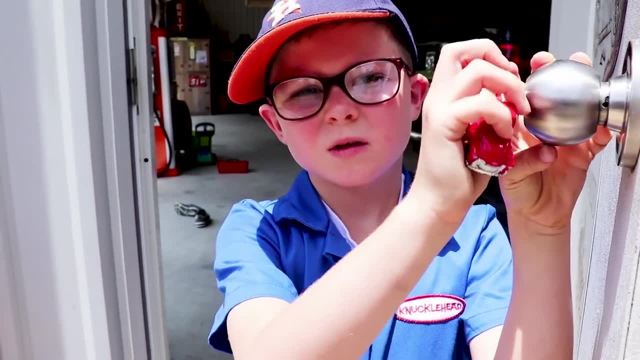 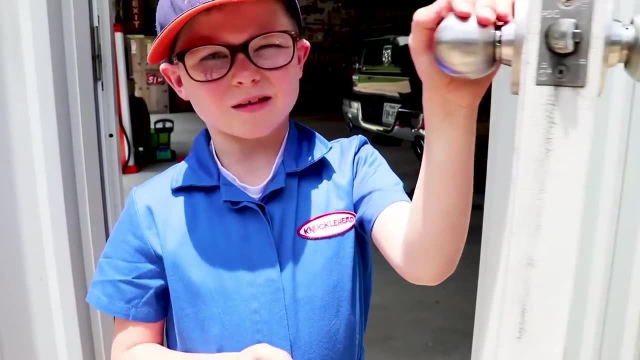 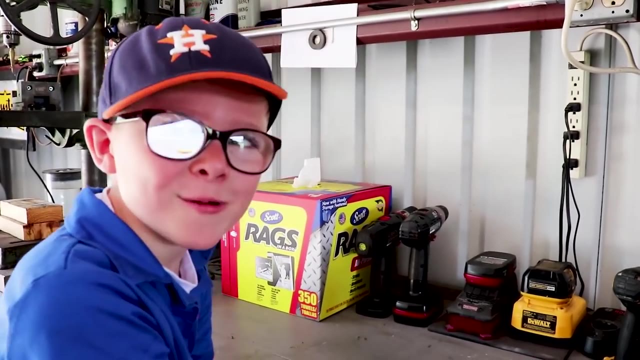 That's not what I really do. I fix real cars. I can make an exception. Let me see what I can do. I think I know what the problem is. Sir, I'm going to need you to step outside while I fix this for you. 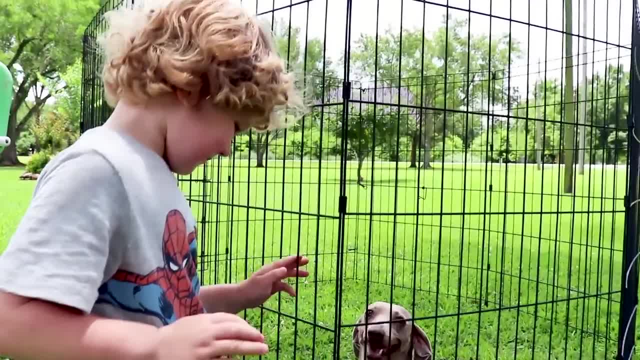 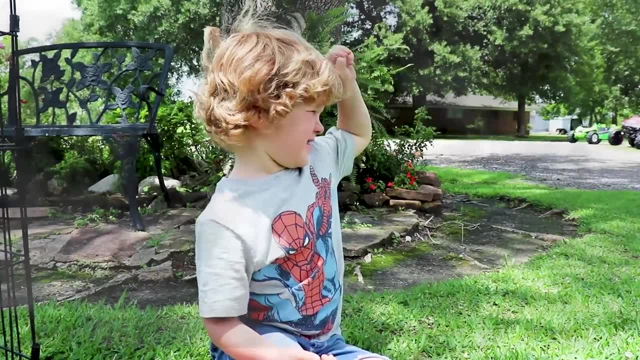 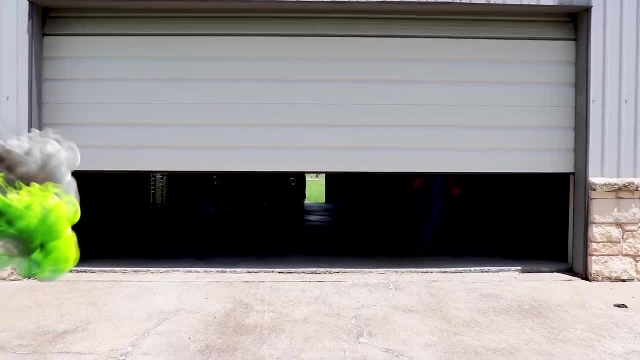 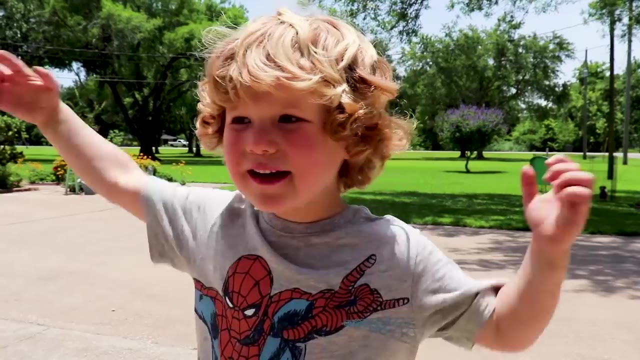 You can go pet my dog, Izzy. Okay, Woohoo, I just played. Hmm, you're in there. I like this shop. Are you ready to see your truck, sir? Oh, I see my truck Here. 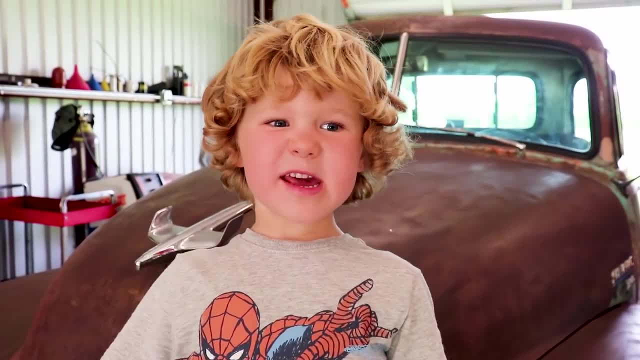 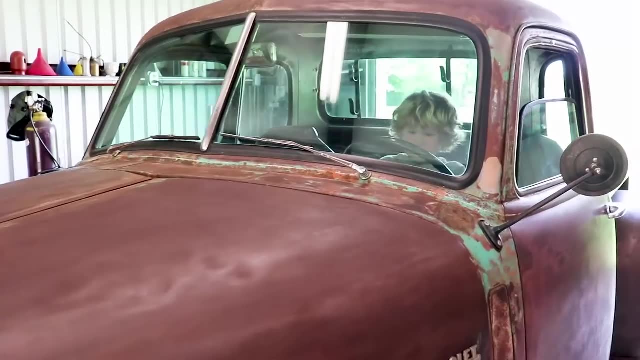 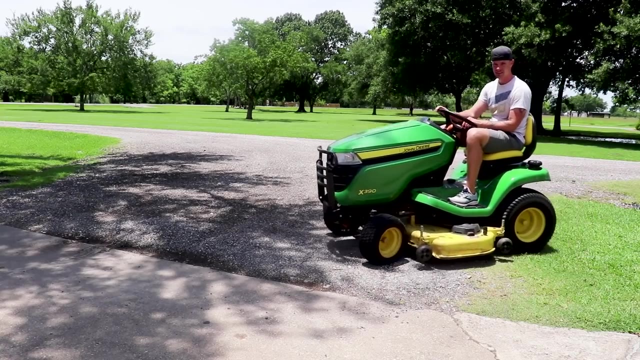 Look, this is my truck. I made it so big. How do you do all this truck? I'm a good mechanic, I guess. Brrrrr, Brrrrrrr, Whee, Are you serious? How did that happen? 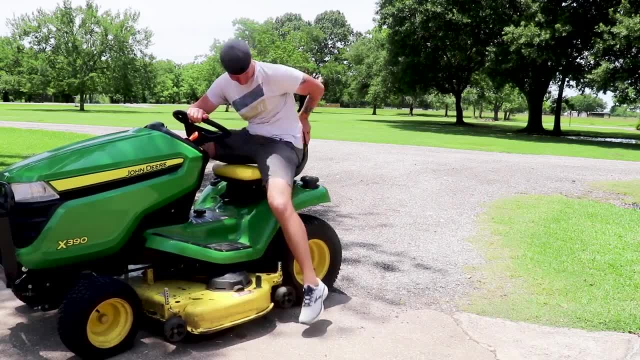 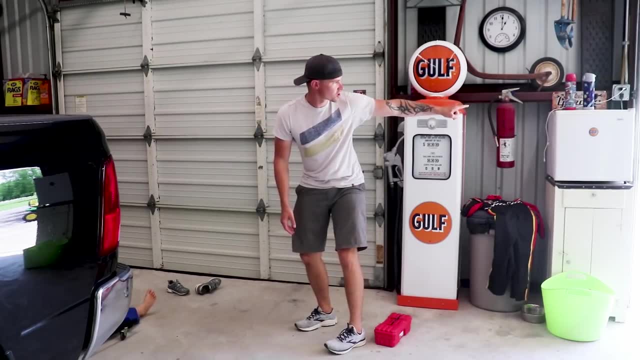 Oh Wonder what he can do to my lawnmower. Sir, Excuse me, sir, Are you under there? Sir, Yeah, Did you really just turn that kid's hotwheel into a big truck? Yes, Uh, my lawnmower's broken. Do you think you can fix it and do the same thing to my lawnmower? Do you think you can fix it and do the same thing to my lawnmower? Do you think you can fix it and do the same thing to my lawnmower? 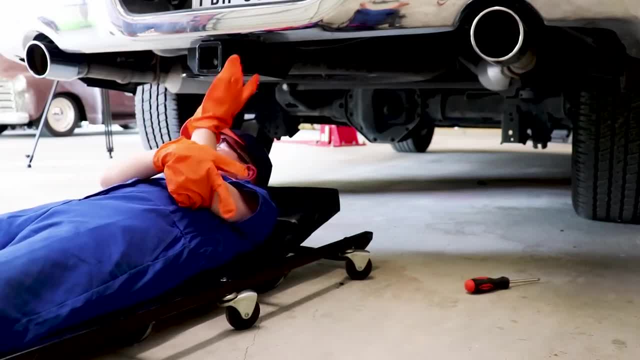 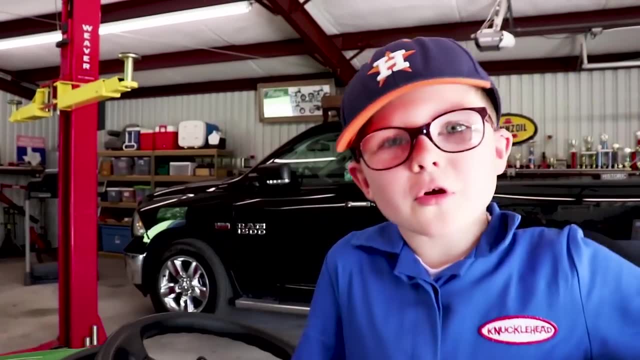 Yes, Yes, Yes, Yes, Yes, Yeah, Yes, Yes, Yes, Yes. a lawnmower? Sure, Okay, come here, I'm gonna show you what's wrong with it. Sir, I need you to go outside while I fix this, please. 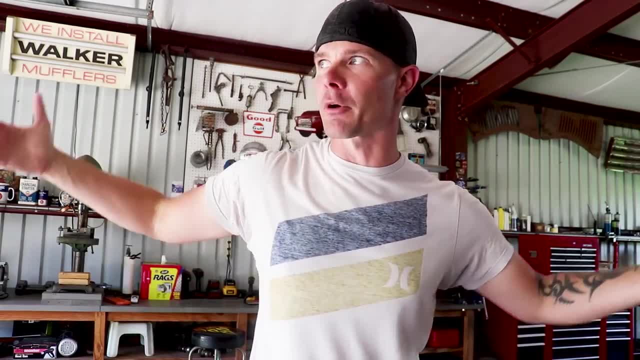 Okay, sir, I'm in a really big hurry. Can you hurry up? I really have a lot. I have a big yard to mow. Yes, you can go pet my dog. Uh, I don't really like dogs, Oh no. 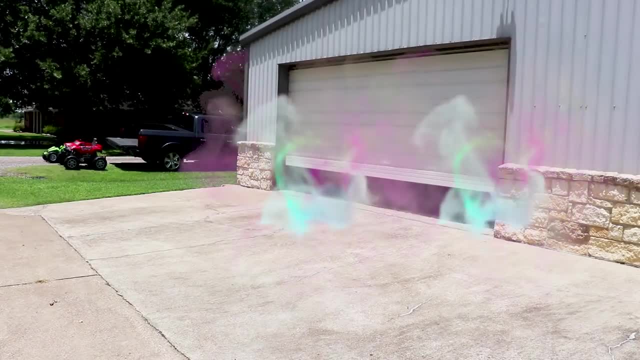 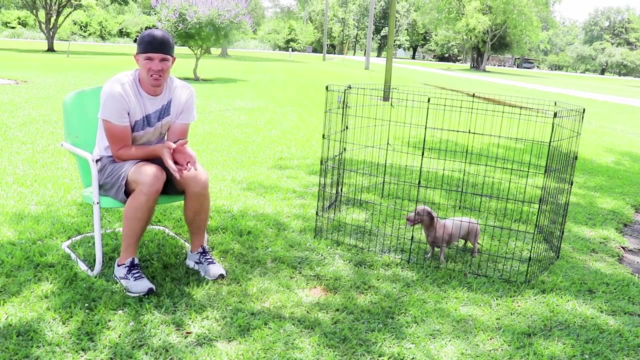 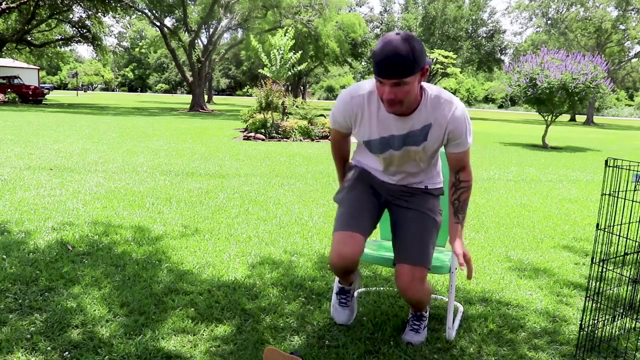 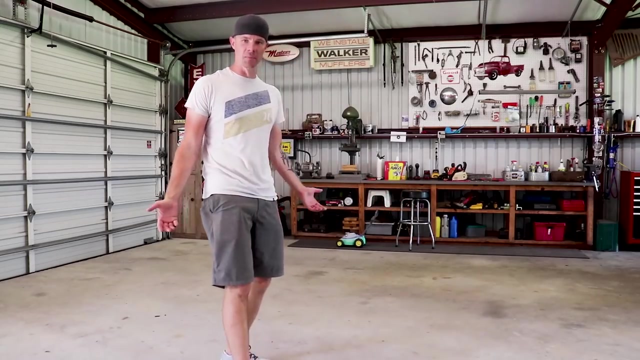 He doesn't like dogs. I don't like dogs. Ah, I don't like dogs. Oh boy, it's ready. Wait, wait. Where's my lawnmower, Sir? where's my lawnmower, It's right over there, dude. 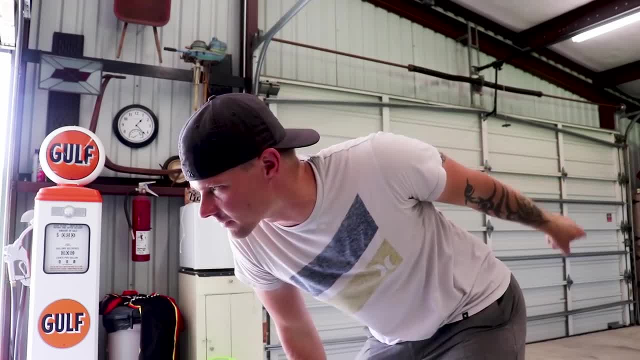 I don't see anything except that little piece of wood. I don't see anything except that little piece of wood. I don't see anything except that little piece of wood. Don't push toy mower over there. That's it. What Are you serious? 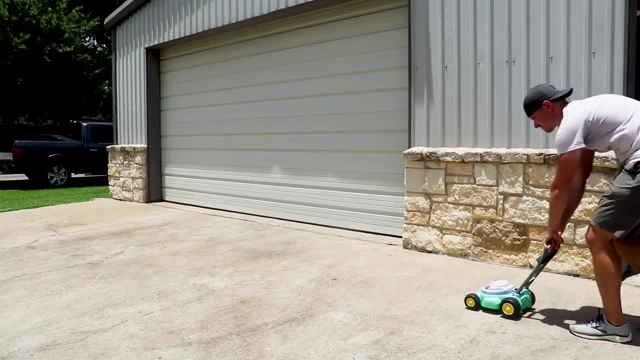 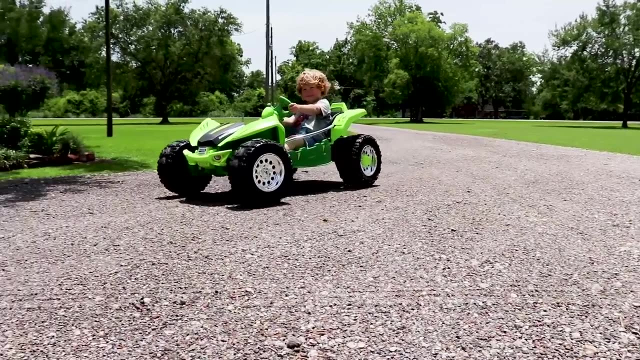 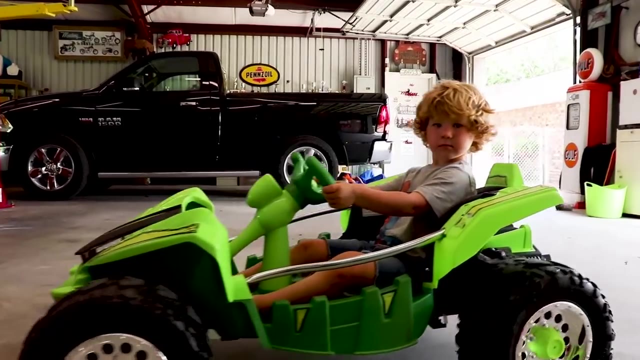 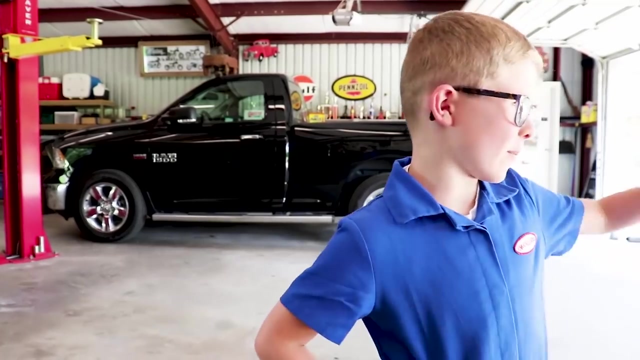 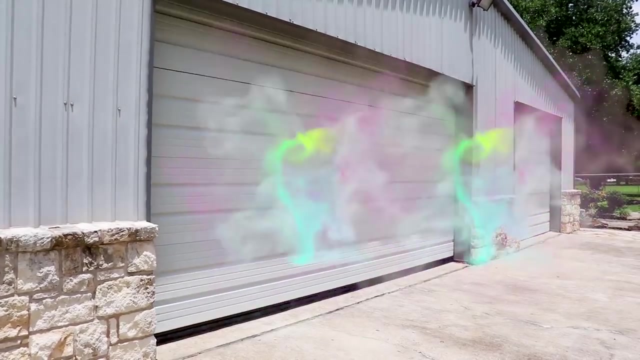 Now please leave. I have work to do. I'll be right there. My dumbbell is broken. Sure, go fix it. I'll sit by my dog while I fix it. Oh yeah, It's a big job to me. 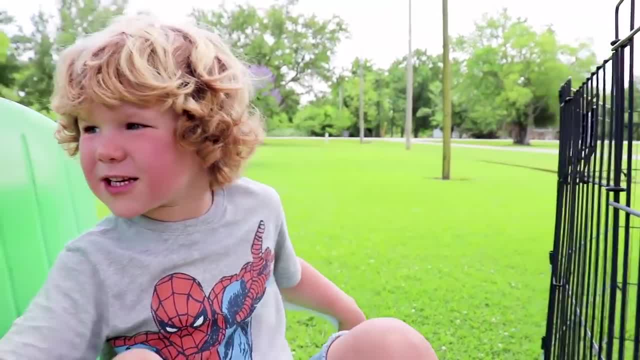 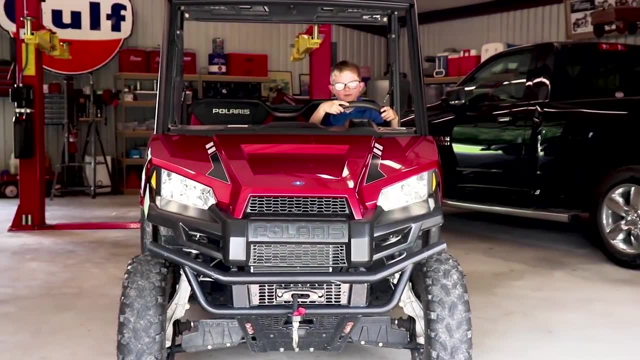 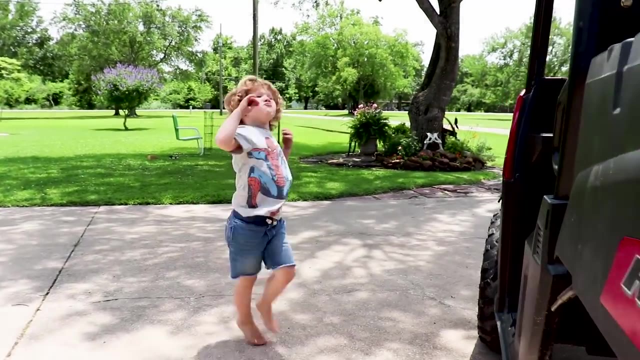 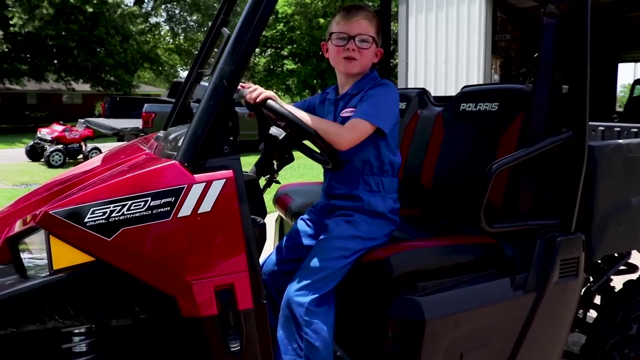 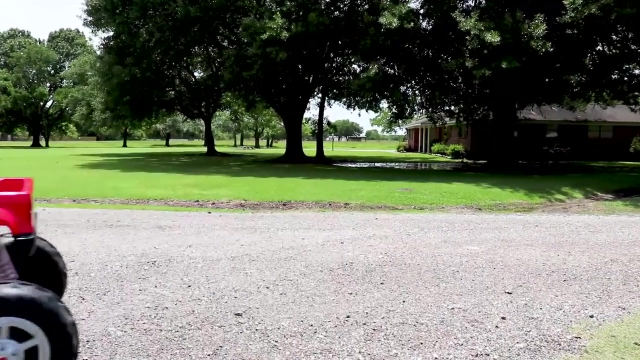 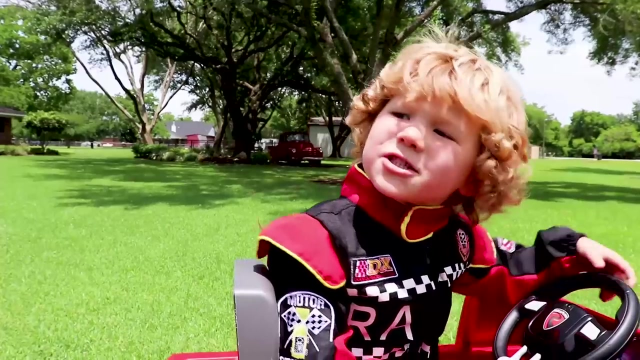 I like this stuff. Oh, my dumbbell buggy is ready. What Whoa? it's big. How do you make it so big? I'm a mechanic, I'm a mechanic. That's what mechanics do. I wish that sound better. take it to the shop. 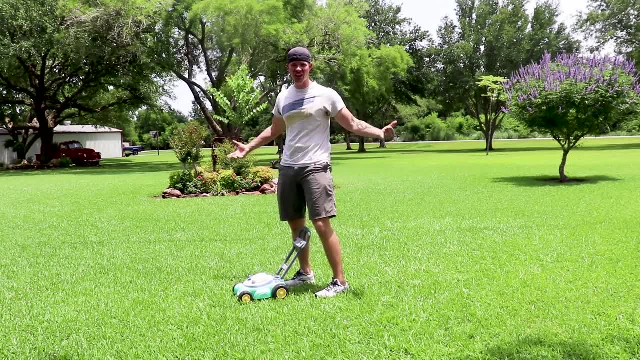 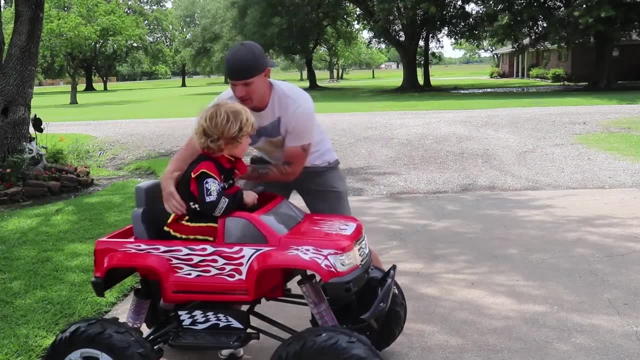 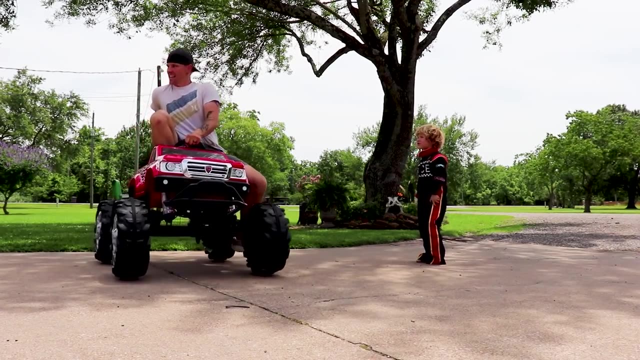 What Are you serious? Try this again. No, that's my monster truck. No, this is my monster truck. Uh, I need to borrow it real quick, please. Thank you, Hey. Hey, Come on, buster truck. 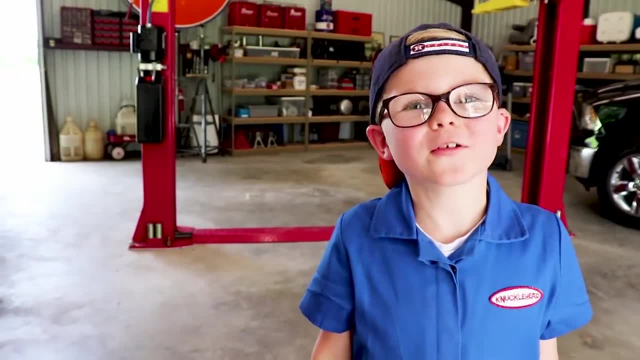 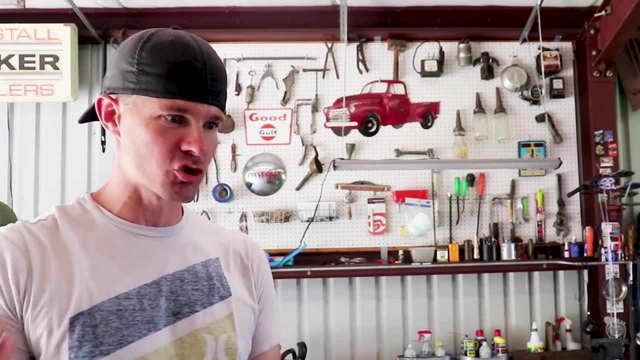 Mechanic, Mechanic, man, where are you? What is it? buster, Listen, I know that you have been taking this other kid's stuff and every time he comes in here you make it super big, But every time I bring something in you make it really small. 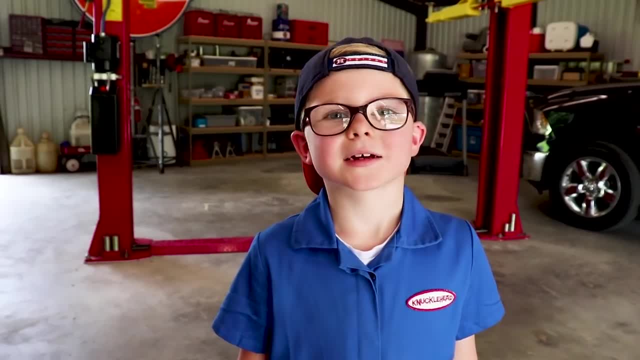 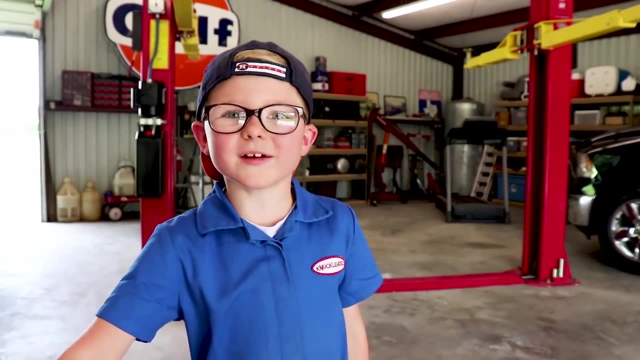 I want this monster truck to be huge. Okay, I'll see what I can do. Okay, so you're saying I'm going to get a big monster truck? No, I said I'll see what I can do. Please wait outside by my dog. 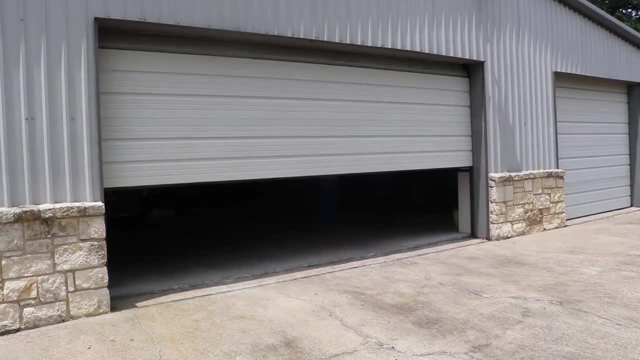 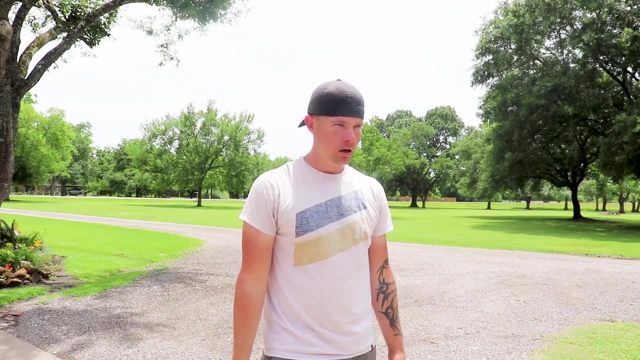 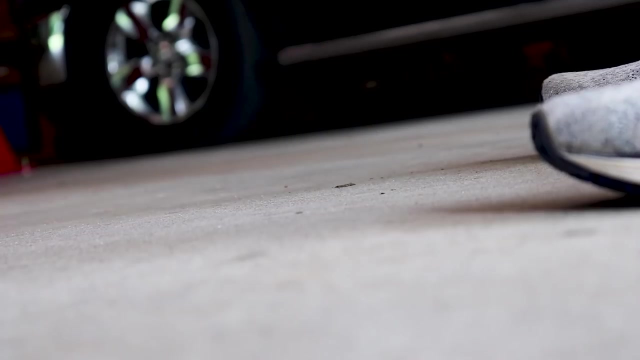 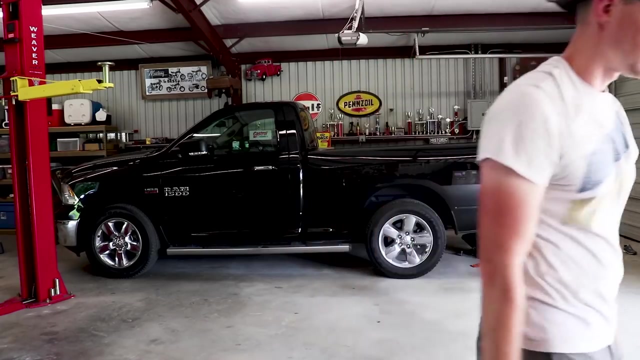 I really like dogs. I can't wait. it's going to be the biggest monster truck ever. Seriously, Bye, I have to go get my lunch break. Your truck is right there. Seriously, Braxton and Ryder are working at the truck. 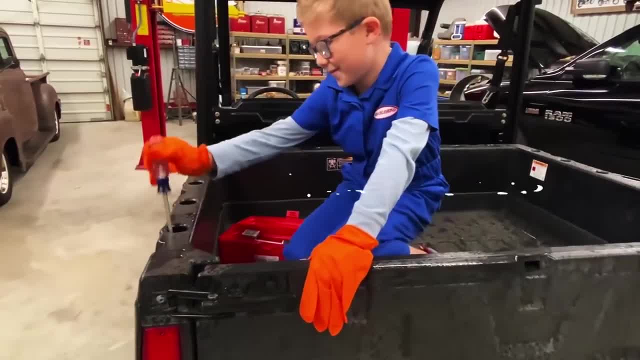 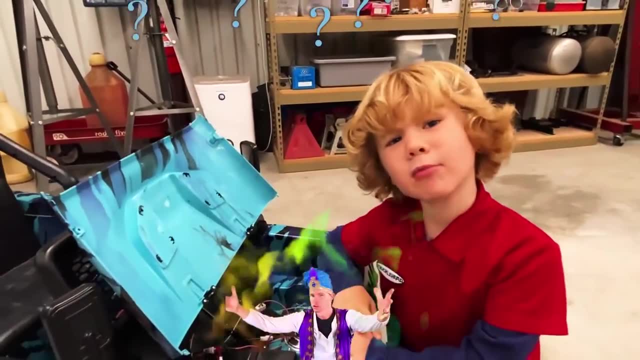 I got to fix this thing. I better fix this rhino, because the owner's going to be here any minute. Ryder has lost his tools. Where is my tool? Oh man, I'm just. I'm going to buy some tools. 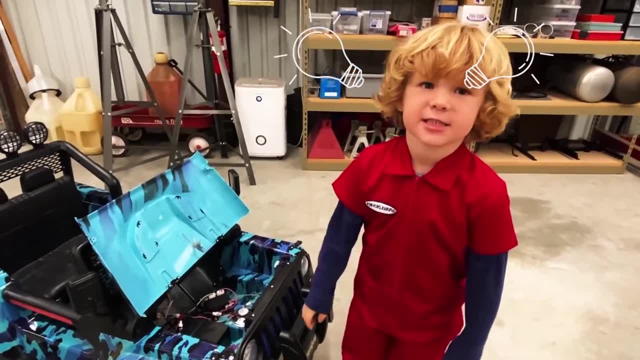 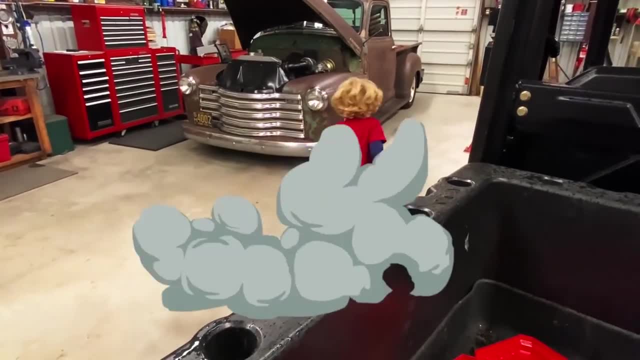 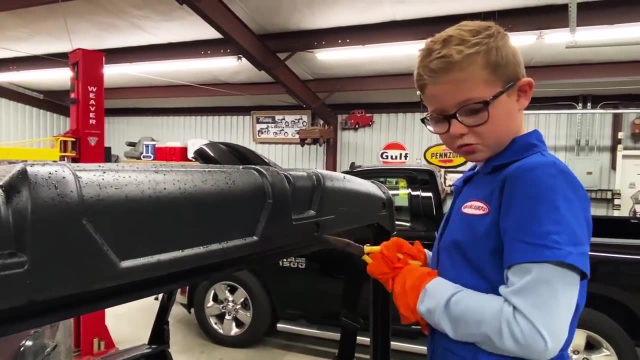 I have an idea. I'm going to get Braxton's. Let's go. Ryder has found a tool. Oh no, Ryder needs Braxton's tool. Braxton needs his tool to fix the truck. Uh-oh, we're in big trouble now. 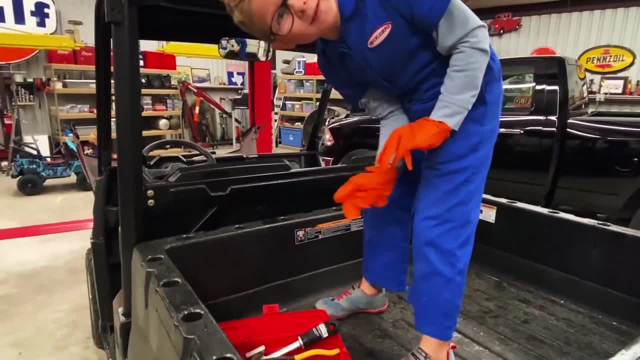 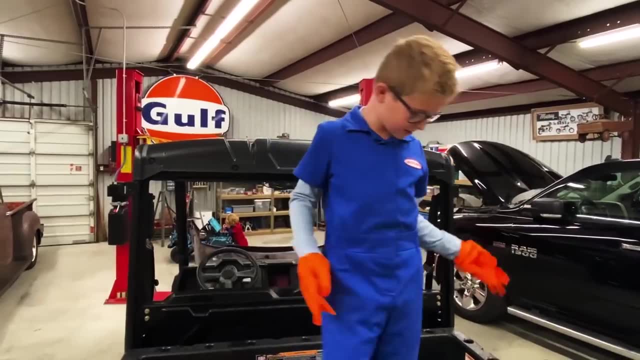 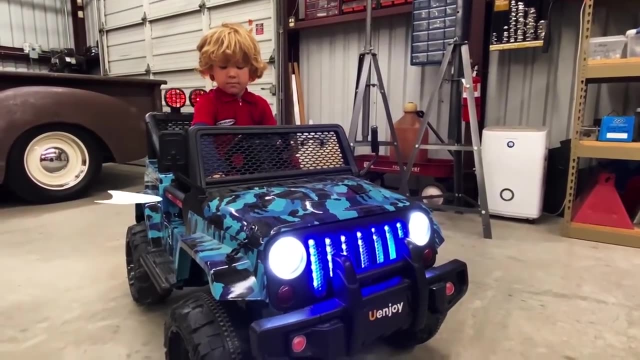 Okay, now I need my screwdriver. What? Where did my screwdriver go? I have to find my screwdriver. I can't fix this without Without it. Ryder has fixed the wheel. I'm fixing it. Yay, Oh yeah, I'll fix. 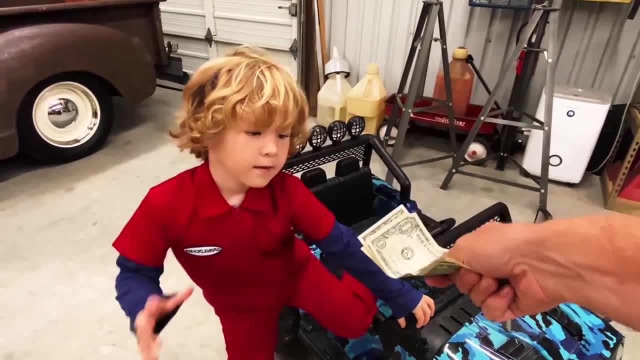 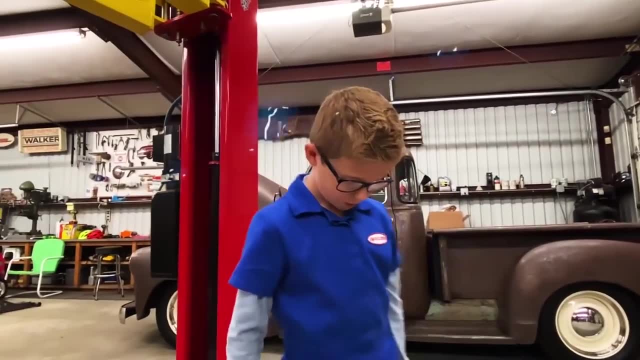 I will teach this fixer. Yay, Yippee, Yippee. Where is my screwdriver? Where Braxton is behind schedule. Ooh, watch this. There it is, But how did it get there? I'm going to forget about that. 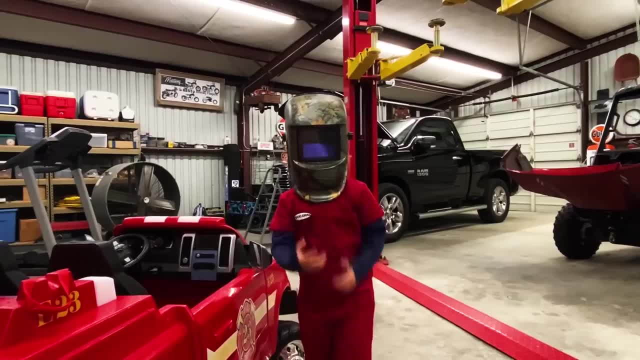 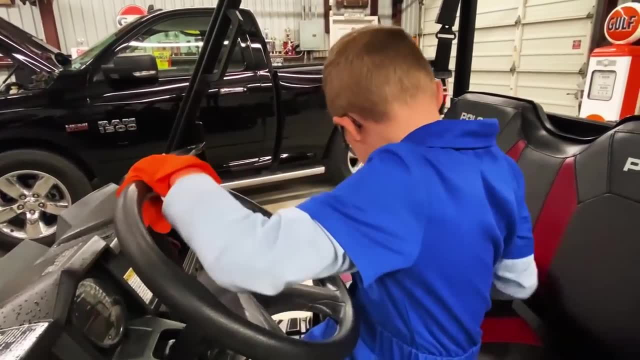 I'm going to forget about that. I'm going to go get my screwdriver. Yeah, I'm just going to go work on that truck. I really have to get this working. Where's my tool? Oh no, Ryder has lost his tools again. 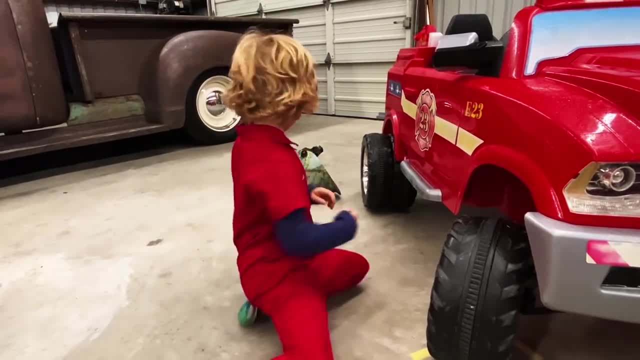 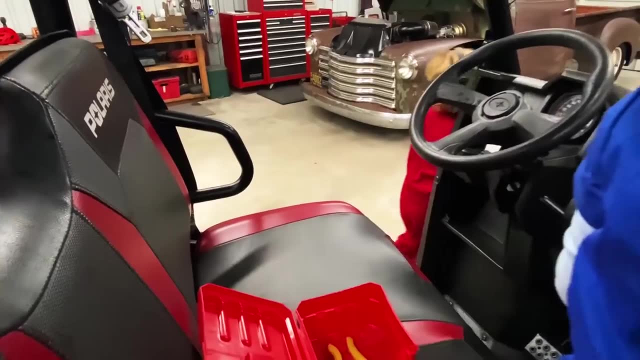 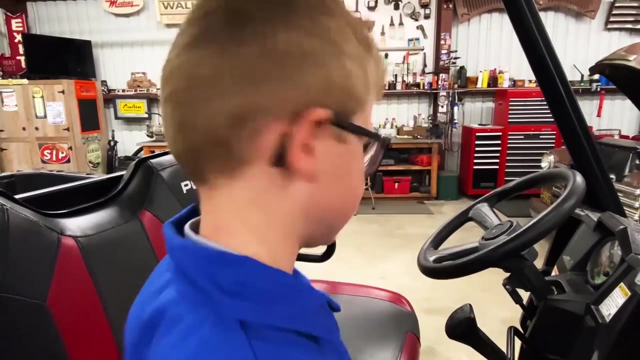 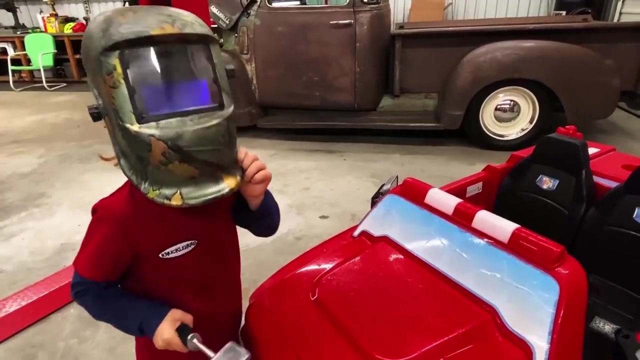 Where is my tool? Where is my hammer? Ryder has found a hammer. Now I need my hammer. Where's my hammer? What I have? all my other tools except my hammer? Ryder has fixed the toy fire truck. Ryder, the truck is finished stop. 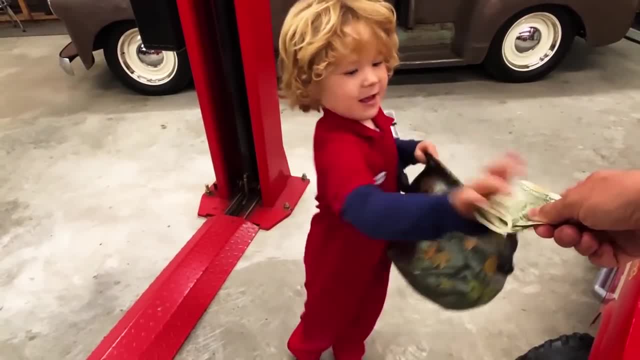 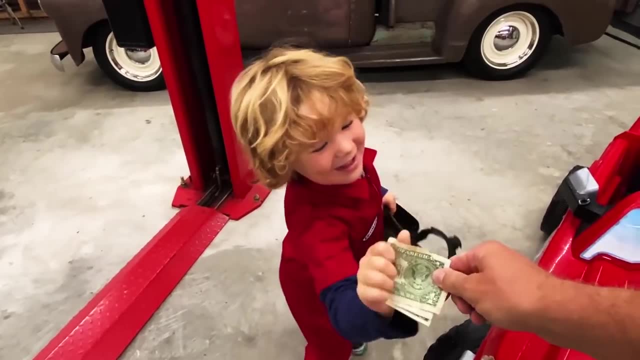 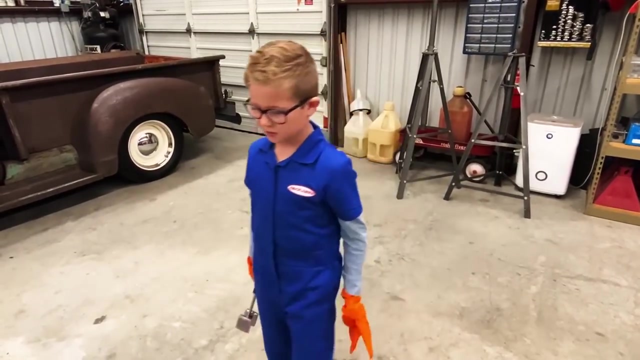 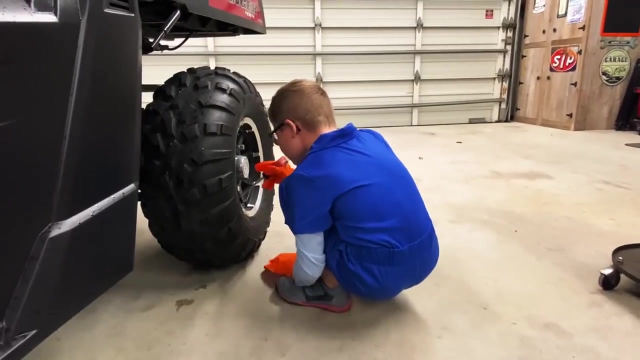 The customer is very happy and pays. Ryder, I can't get this on. Braxton is very, very late. How do my balls keep getting right here? Braxton has found his hammer, My leg's sore. I need a stool. 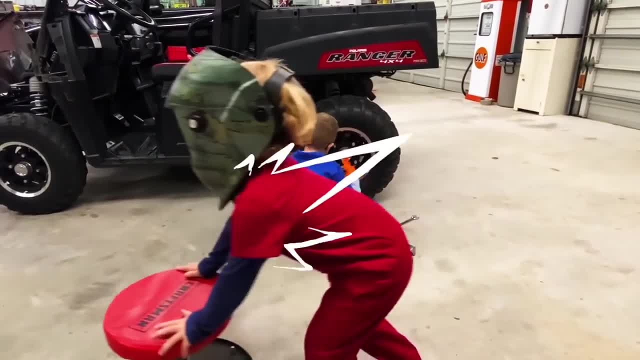 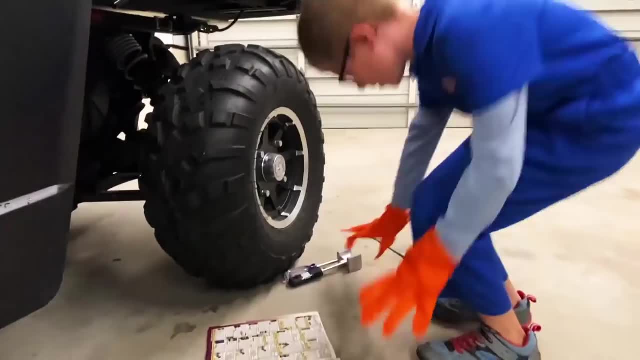 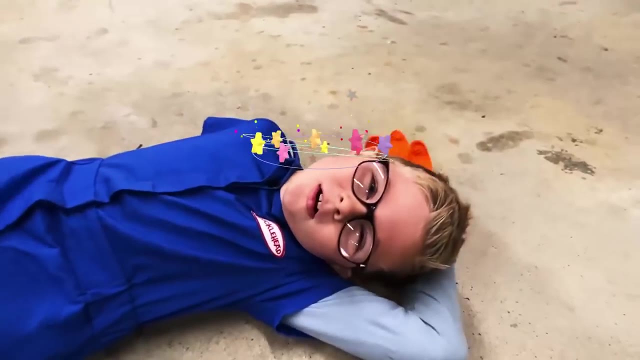 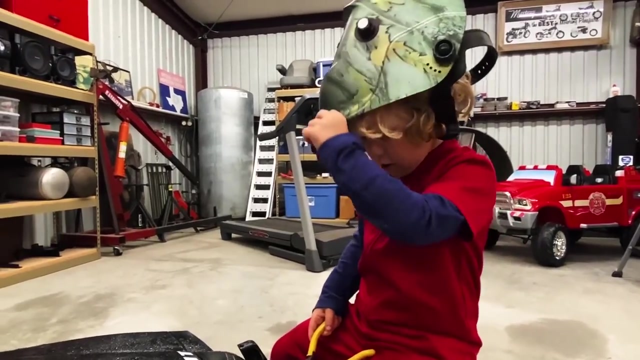 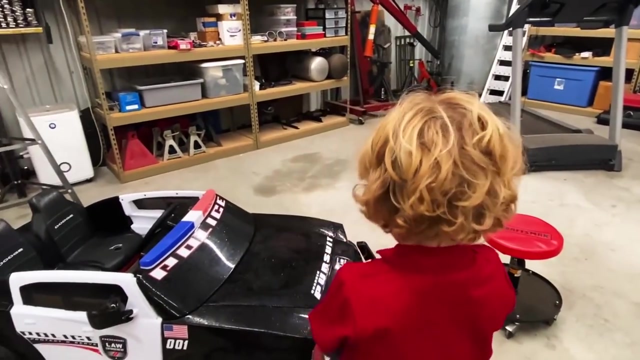 The rider has taken Braxton's stool. I need my stool. He stole my stool. Rider is playing on Braxton's stool. Rider has fixed another car Because finish saw. Yes sir, Uh-huh, Yes sir. 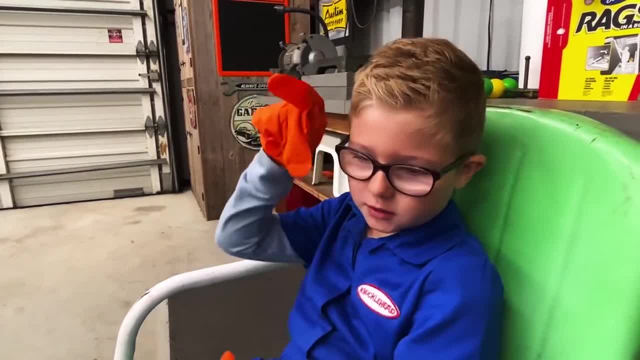 Yes, sir Braxton's boss is now happy. He said: if I don't finish this car today, I'm going to be in trouble. I'm going to be in trouble. It's fire, Braxton, I'll help you fix it. 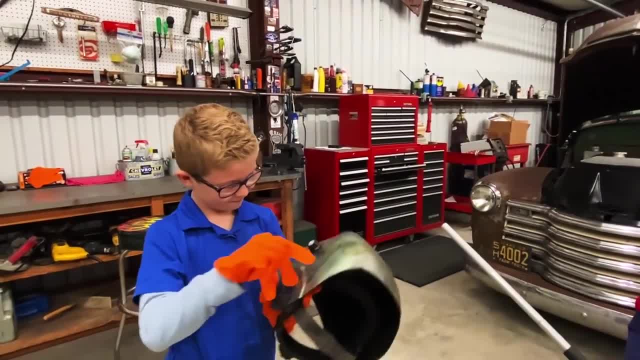 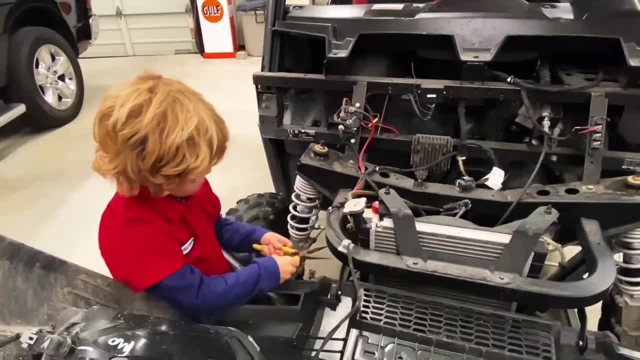 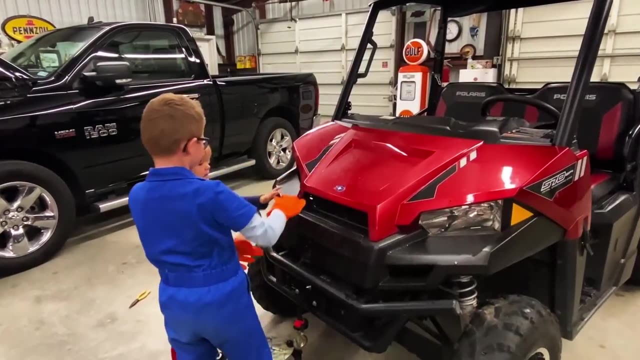 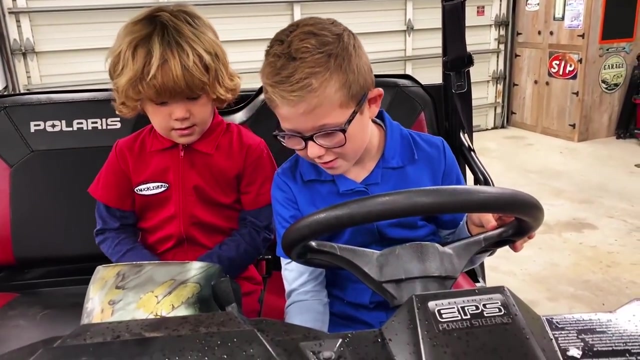 You got to have the helmet. Okay, Rider shares his helmet with Braxton. Braxton and Rider have fixed the truck. Let's install this and see if it works. Okay, All right, Sir, your ranger is done. Thank you. 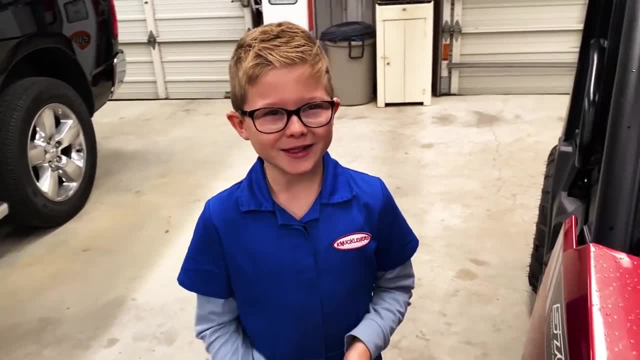 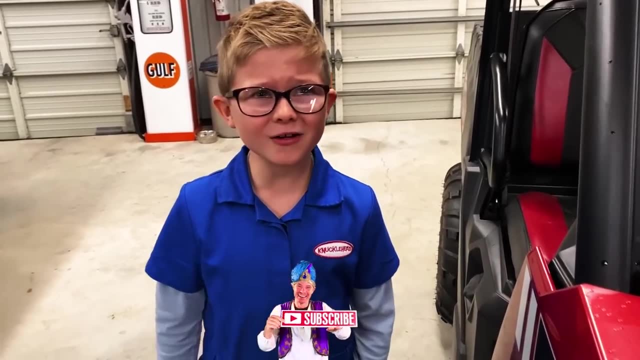 Have a nice day. Everyone subscribe and like and hit that bell. If you want to see more workman videos, go on our Instagram and tell us Bye, Bye.